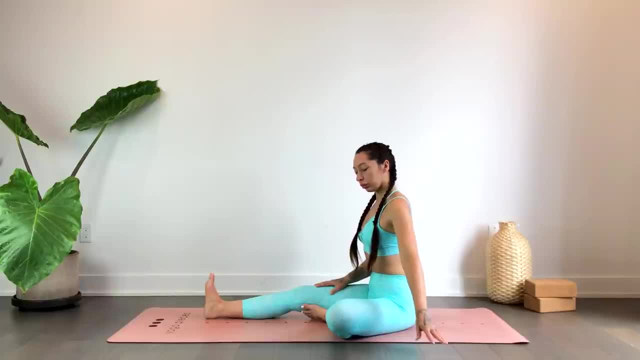 your left hip, maybe even coming down to the elbow. Inhale right hand reaches up for a gentle side stretch, opening that right shoulder. Take your gaze up. Inhale side stretch towards the right Again. feel free to come down to the elbow if the body allows it. 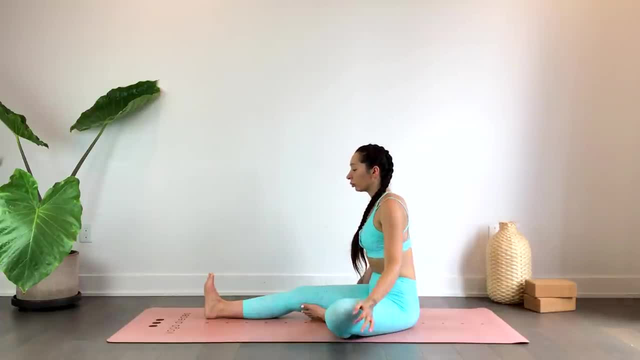 Inhale, come all the way back up and we'll go ahead and hinge at the hips, leading with the chest folding forward, stopping wherever you feel the stretch. You'll notice I'm not folding too deep into this pose because right here is where I need to be. 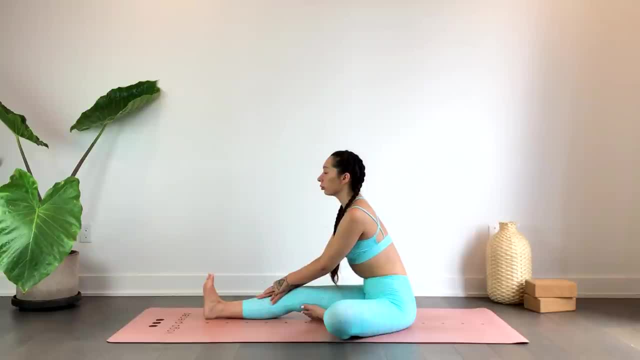 today. That is where I'm feeling the stretch, so I'm going to stop right there, Listening to the body, keeping that nice neutral spine, Drawing the breath into the belly, into the lower back, expanding the waistband of your pants with each inhale. 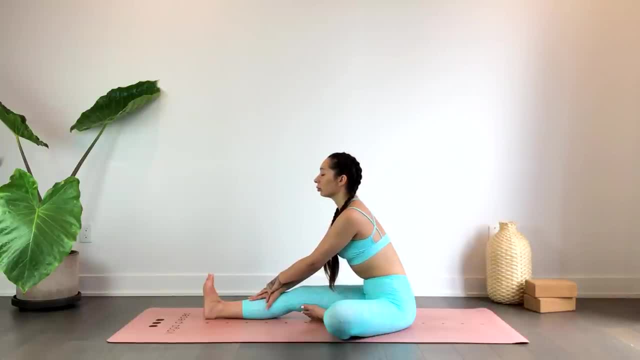 Maybe with each inhale you're going to feel the stretch. Maybe with each inhale you're going to feel the stretch. Maybe, with each inhale you're going to feel the stretch. Maybe with each exhale have the intention, even if it's just mental, to fold a little deeper. 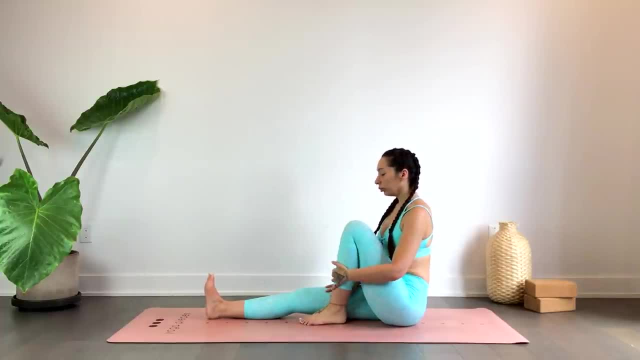 And we'll gently release, Lifting the left knee. we'll plant the left foot to the inside or outside of the right leg, Sitting up nice and tall. once again, feel free to plant the right hand to the outside of the left knee, Left hand just behind you, for a gentle twist as you exhale Or inhale. 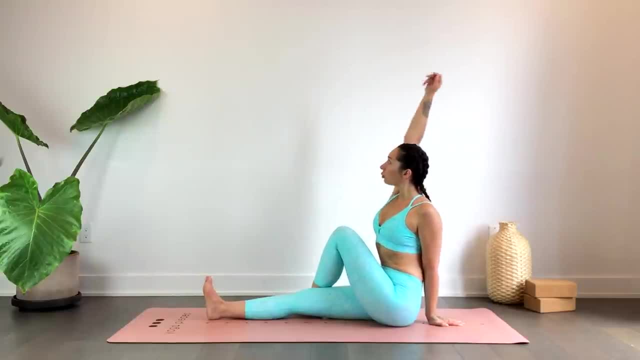 right hand to the outside of the left knee. Right hand reaches up- Exhale, taking that elbow to the outside of the left knee, taking your twist Inhale to sit tall, lifting through the sternum Exhale- soften the shoulders. 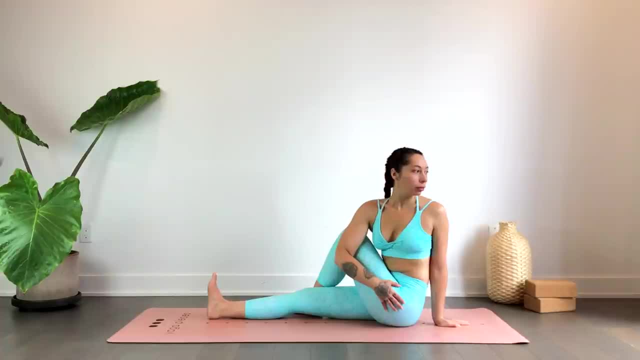 Med 9. We're going to take a break, But don't stop here. Inhale, nehmen Exhale, turn to the rightrue and lift both ankles. come up我就 Exhale of the left knee- comfortable lie down. 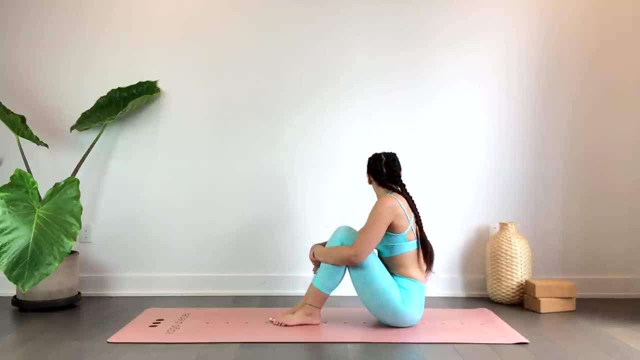 Bend the right knee, pushing your upper tight as you breathe in, And when you're ready, we'll switch sides. So just straightening the left leg toes up towards the sky, Bending the right knee and just allowing that knee to fall open. 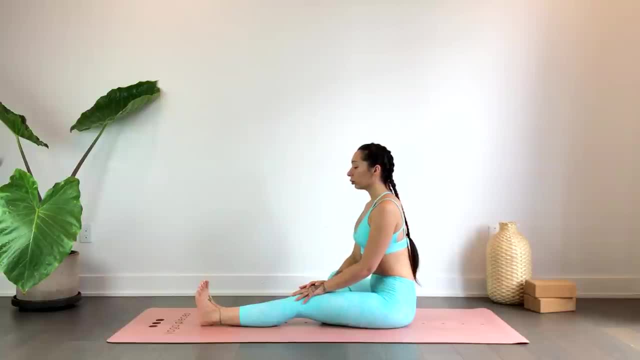 Removing the flesh from your seat. so you're nice and grounded through the sit bones, Sitting up tall. go ahead and take a side stretch towards your left. Right hand reaches up. Inhale back to center. Exhale side stretch towards your right. 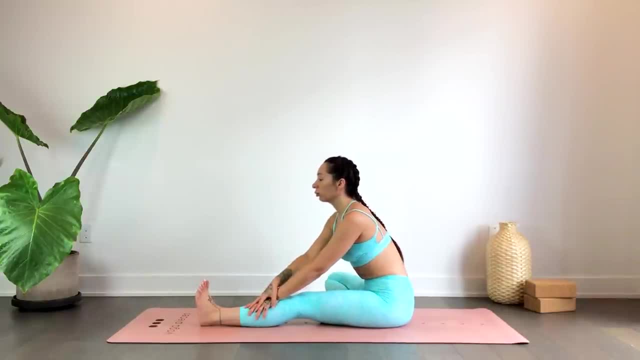 Inhale, come back to center, We'll go ahead and take our forward fold. So just folding and stopping wherever you feel the stretch, Avoiding any rounding throughout the spine as much as possible. Again, it's not how deep we can go in the pose. 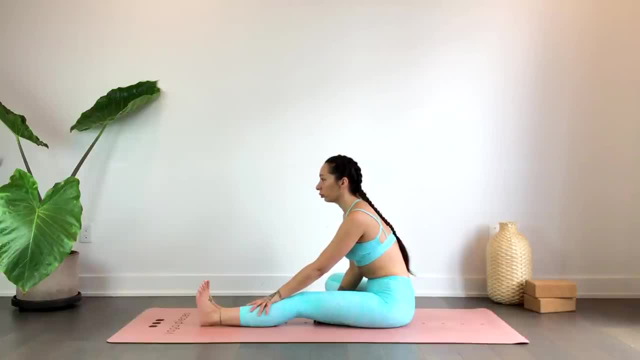 It's just about how we feel, right here and now, And we'll go ahead and release, lifting that right knee And again just planting the foot on the inside or the outside of the left thigh, Left leg, Inhale to lengthen. 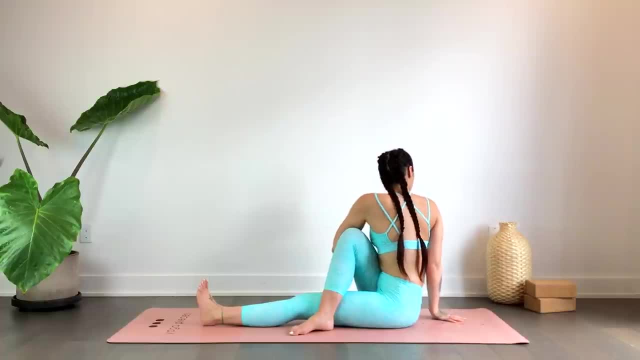 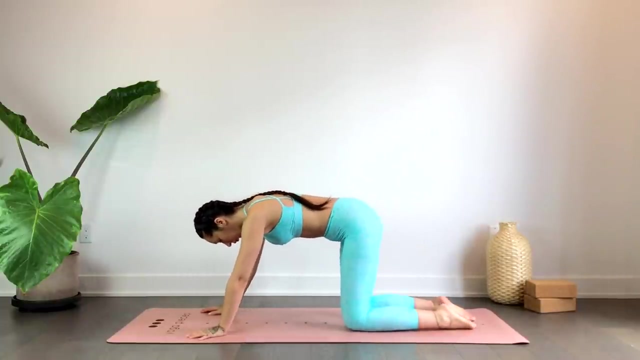 Exhale to take your twist. Thank you for watching. Take a moment and we'll meet in tabletop. pose wrists under shoulders, knees under hips- We'll inhale, dropping the belly. Take your gaze up for cow pose Exhale, rounding through the spine. 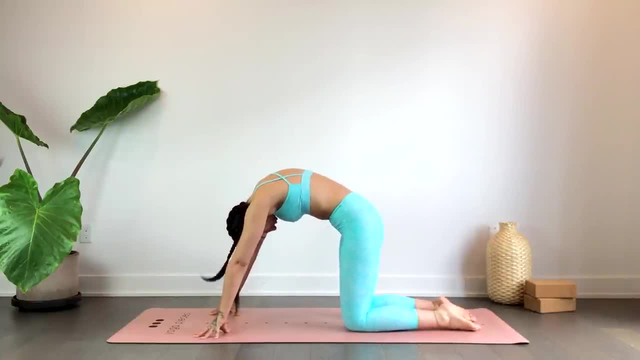 Take your gaze down for cat. Continue sinking breath with movement flowing at your own pace. Take a moment and we'll meet in tabletop pose, wrists under shoulders, knees under hips, Finding a neutral spine. we'll begin to walk the hands forward, keeping the hips just above the knees. 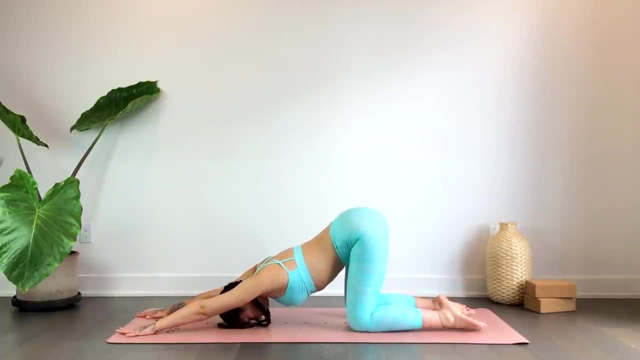 As you melt the chest and forehead down towards the mat. Feel free to place a block underneath the forehead for added height and support here. Just taking a moment to observe the body, observe the stretch On your inhale, rounding through the spine, coming all the way down to your belly. 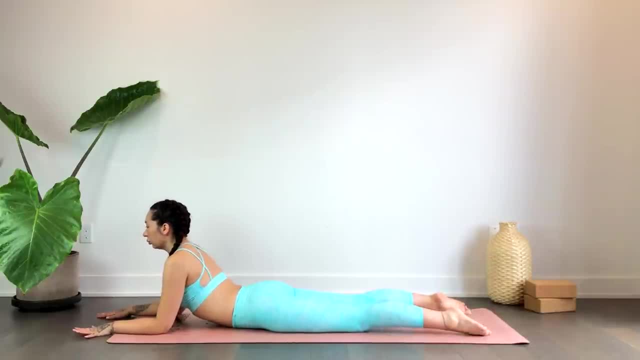 Just lifting on the forearms, tucking the tailbone, and just lifting through the sternum here, Softening the shoulders away from the ears, maybe begin to find some movement, Rocking side to side, gazing over one shoulder, then over the other. 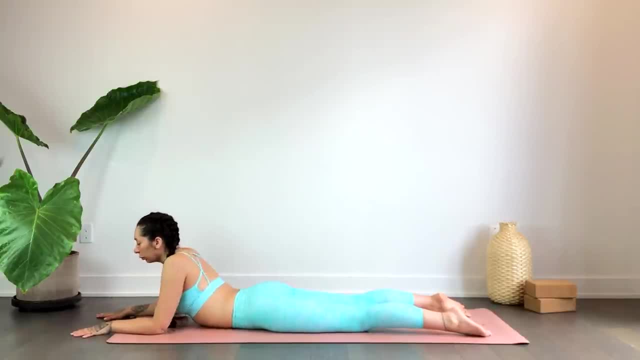 now you can stay right here, find any pose that feels best for you, or you can try this next pose. it might be a bit intense for many, so do listen to the body. skip it. if it doesn't feel right today, we'll come all the way down to our. 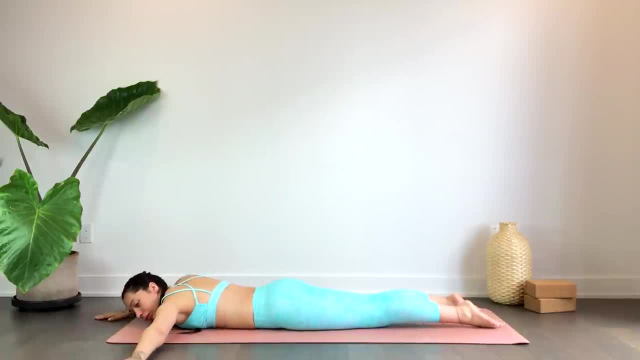 bellies, and we'll take the left hand straight out towards the left side so that the wrist is in line with the shoulder, staying right here if this is enough of a stretch- and it will be for many. so do listen to the body once again. if you'd like to go a little deeper, open up the entire body towards the right. you. 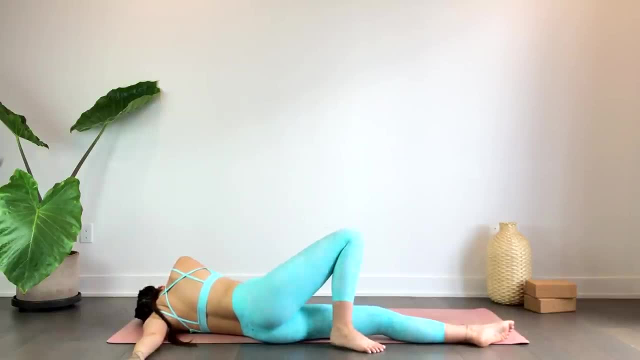 can take the right foot to the inside or outside of that left leg, or you can drop the knee down, so resting the right ankle just above the or on top, rather, of the left thigh, using your right hand as a bit of support here again, staying wherever you feel most comfortable. 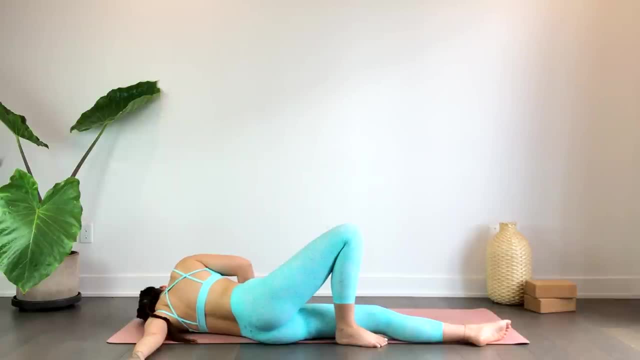 observing more, reacting less, and we'll gently release. take a moment whenever you're ready, we'll switch sides. so just straightening the right arm out towards the right, you can see right here- begin to open up towards the left left foot to the outside of the right thigh, or you can drop that knee. 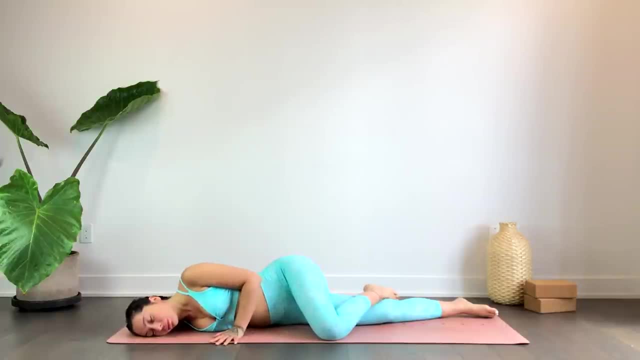 once again using the left hand as a support here. you can do the other side with your right and you can do the other side with your left foot through the right foot and warm, put it up to the back on the leg. do Ri Je On Fe Can. 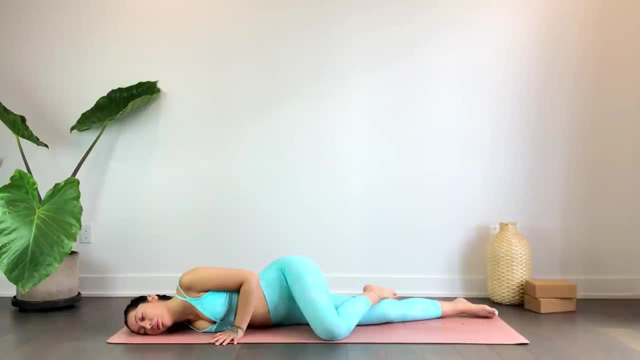 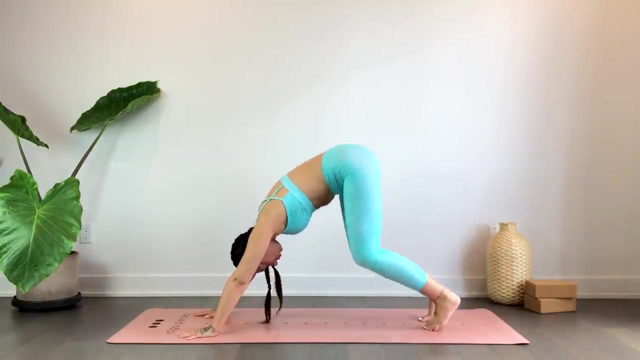 We'll gently release, take the hands to your sides, just taking a moment here to completely let go. Then we'll meet in down dog, whenever you're ready, sending the hips nice and high, keeping a bend in the knees, maybe, walking one leg, walking the other, pressing the mat away from. 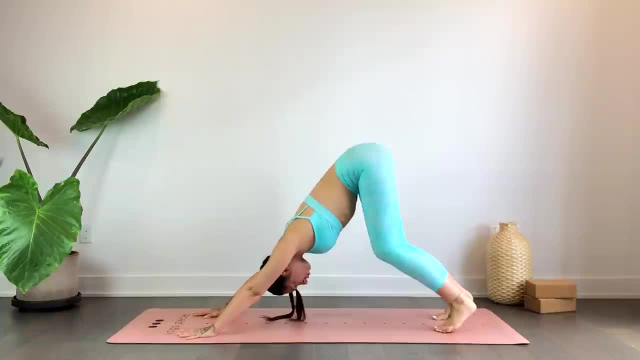 you Engage the entire body here. Good, And as you exhale, plant the knees, sending the hips towards the heels, forehead or cheek to the mat for child's pose, Taking a moment here of rest just to kind of observe the body and just soak in all the.